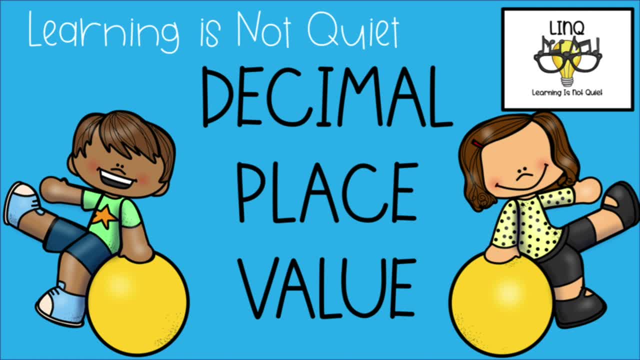 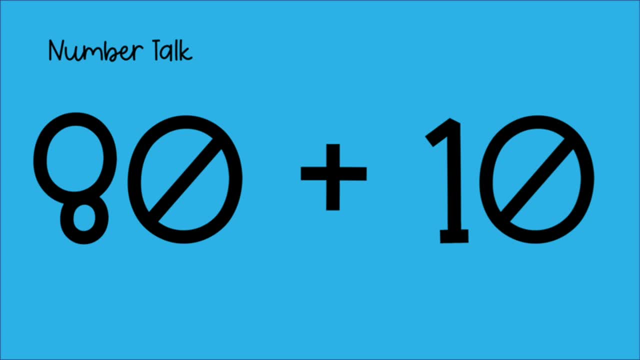 you're curious about or need to work on. You're doing great. Let's get started with our number talk. Let's take a look at this question first. Think to yourself: what is the answer to 80 plus 10?? If you said 90, you're correct. You could have. 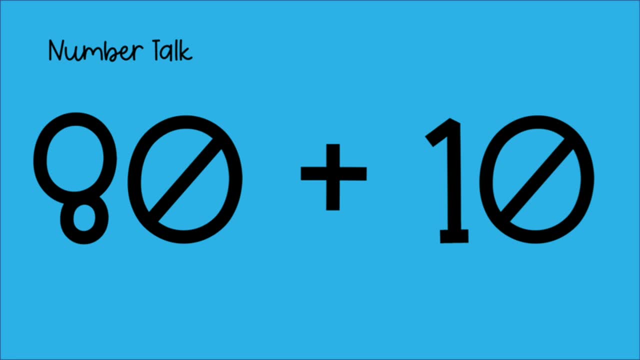 done this by counting up from 80,, 81,, 82,, 83,, 84, and so on to get 90. You could have stacked them on top of each other and added them like an algorithm, or you could have visualized base 10 blocks. I bet you can use that same line of thinking to. 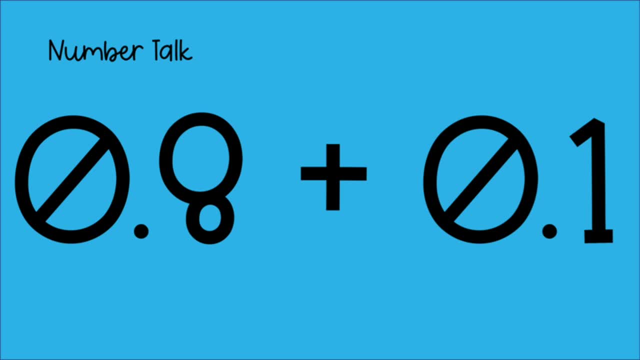 answer this question. 8 tenths plus 1 tenth is what? Take some time and think of as many strategies as you can to answer this question. Take your time, Remember you can always pause this video, especially if you're writing a beautiful paragraph on all of your different strategies on your worksheet. There are a 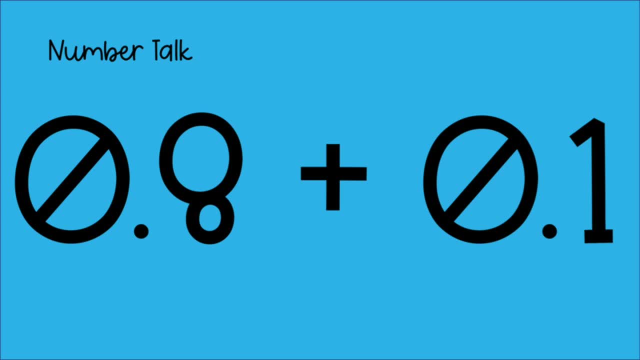 couple different ways we could solve this. We could use 8 tens plus 1 ten equals 9 tens to figure out that 8 tenths plus 1 tenth equals 9 tenths. We could also think about this like money: 8 dimes plus 1 dime equals 9 dimes or 90. 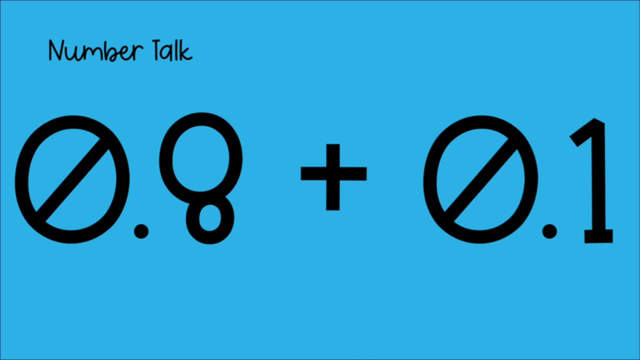 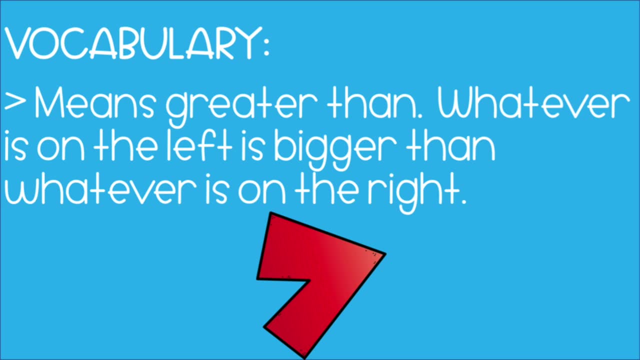 cents. You might also know how to use the algorithm where you stack these numbers on top of each other and add them to get 9 tenths. Now let's move on to some vocabulary. This sign that you see means greater than Whatever is on the left. 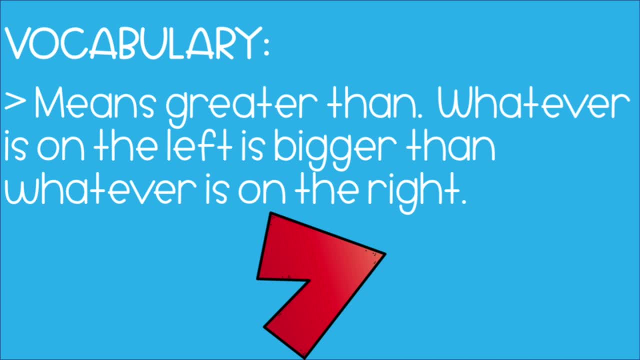 is bigger than whatever's on the right. We often say that it looks kind of like an alligator mouth and the alligator wants to eat whatever number is bigger. Now we see that this sign means less than Whatever's on the left is going to. 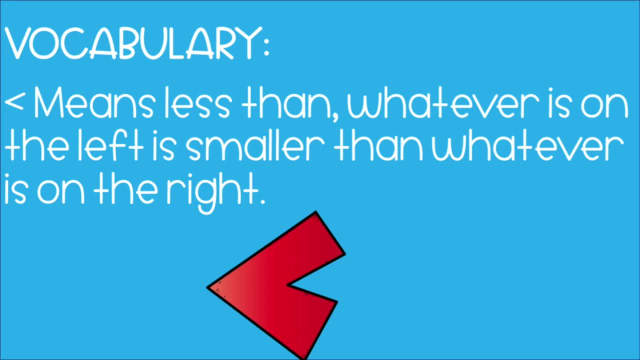 be smaller than whatever's on the right. Sometimes students can get confused with these two symbols, Just like any word or number that we read in English. we read it from left to right, So the smaller part comes first. That means it's less than If the bigger part comes first. reading left to right, that means 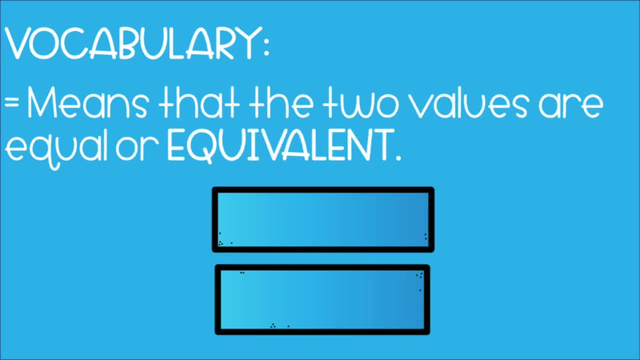 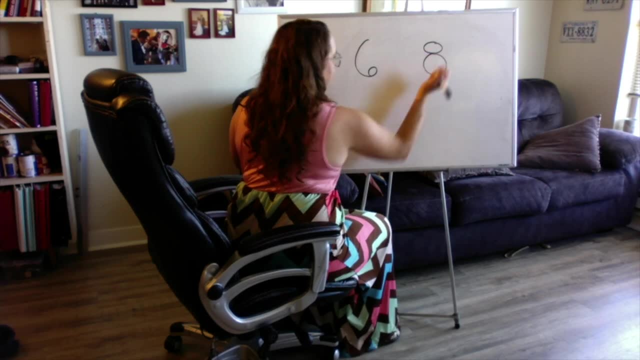 it's greater than. Finally, we have equal to, which means that the two values are the same, equal or equivalent. Let's take a look at the whiteboard. We're comparing the numbers 6 and 8.. 6 is less than 8.. Our alligator wants to eat the bigger. 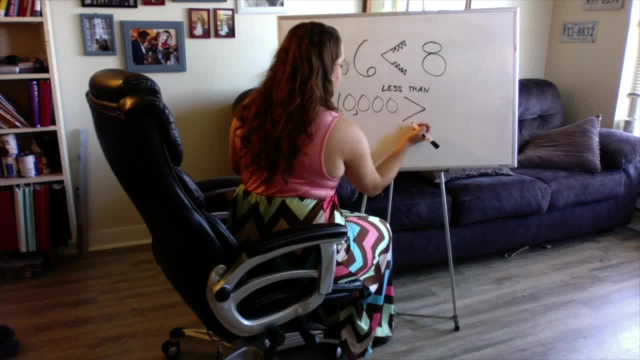 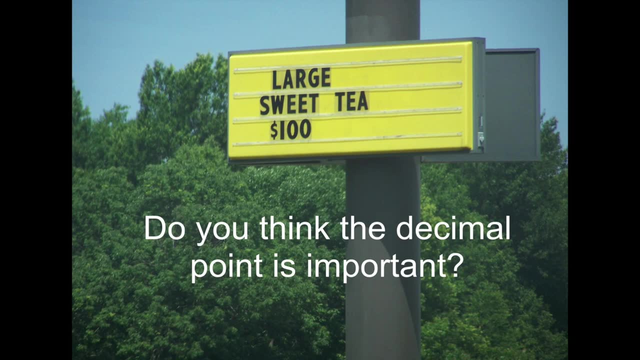 number, and we're reading it left to right. Likewise, 10,000 is greater than 1,000.. That alligator eats the bigger number. As you can see here, decimals are kind of a big deal, What? So, before you spend a hundred dollars on sweet tea, let's understand. 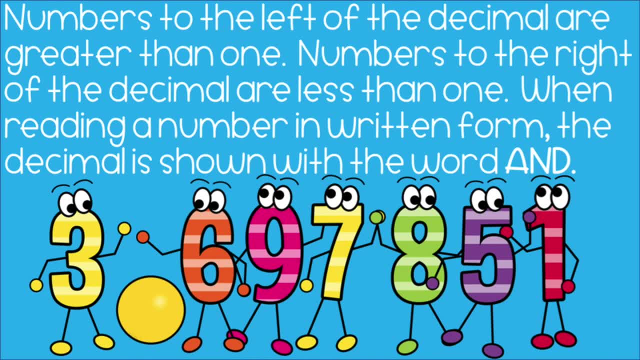 this, Numbers to the left of the decimal are greater than 1,, like the 3 in this number, Numbers to the right of the decimal are less than 1.. When reading a number in written form, which we talked about before, is with words: the decimal. 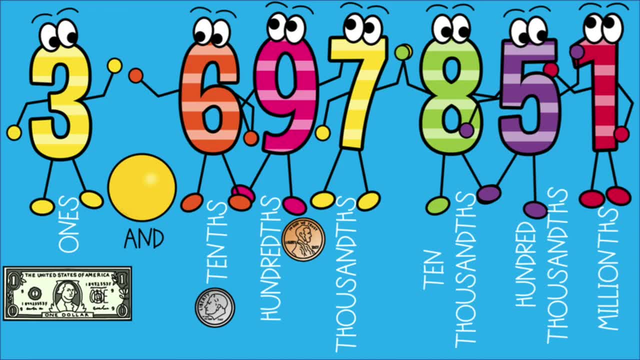 is shown with that word, AND You're probably going to notice that decimal place value names are very similar to whole number place value names, with the exception of this N named FFFF. I am a proud spitter when saying place value names, Hey. 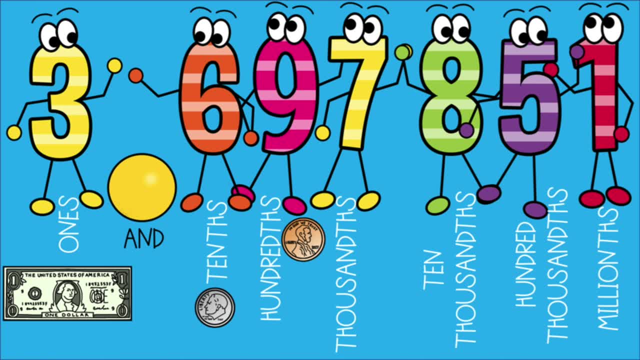 Those number names are ones, and then our decimal, AND tenths, hundredths, thousandths, ten-thousandths, hundred-thousandths, millionths, and so on. Let's memorize these with a chant. looking at this particular number, that 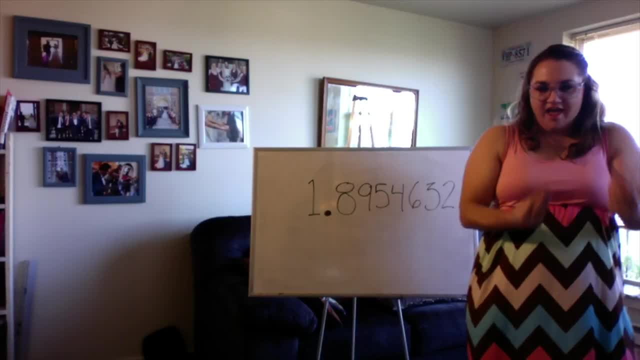 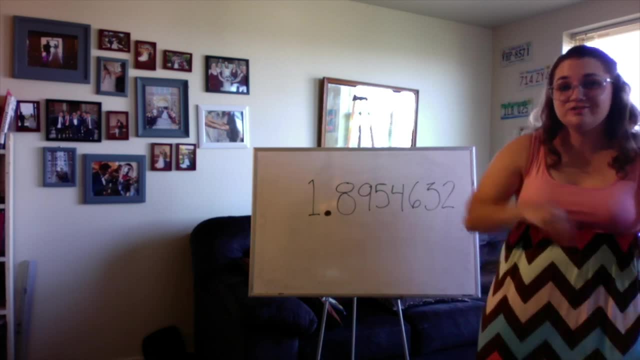 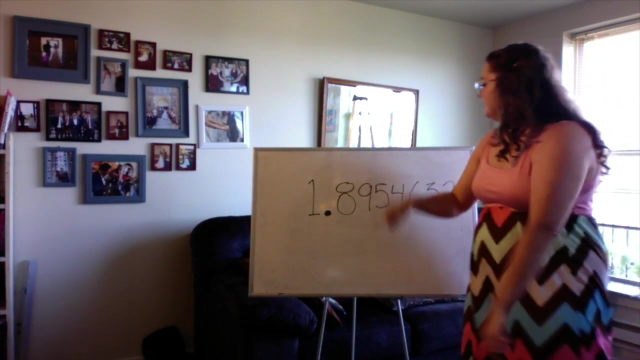 I'm writing on the whiteboard. We started our decimal with: AND tenths, hundredths, thousandths, ten thousandths, hundred thousandths, millionths, ten millionths, hundred millionths, and so on. So eight tenths nine hundredths five thousandths four, ten thousandths, six hundred. 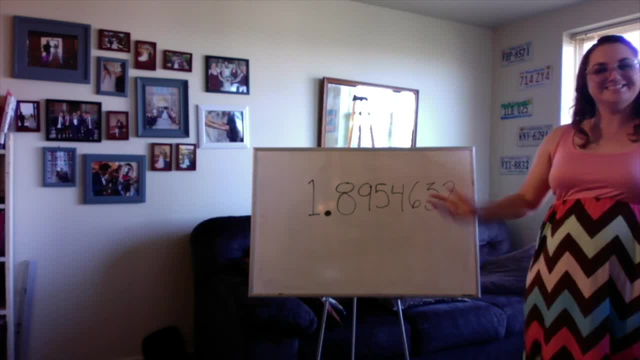 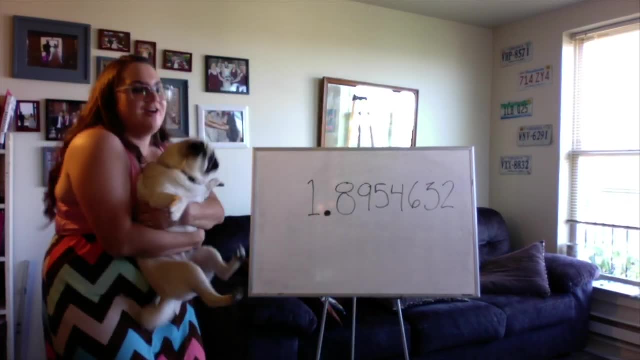 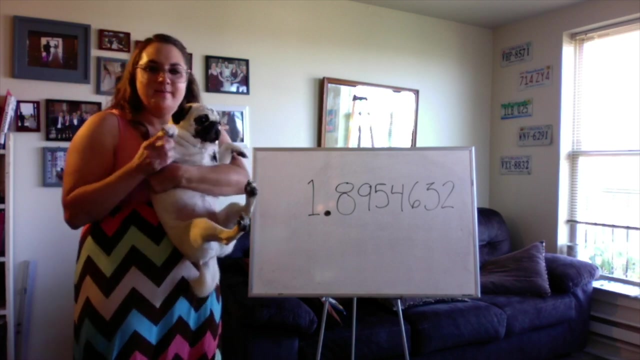 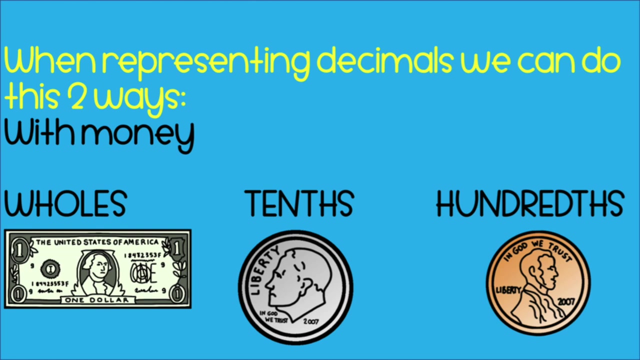 thousandths, three millionths. two, ten millionths. Sing with me and the puppy. And tenths, hundred thousandths, ten thousandths, hundred thousandths, millionths, ten millionths, hundred millionths, Bye, bye. When representing decimals, we can do this two ways. one is with money. Holes would. 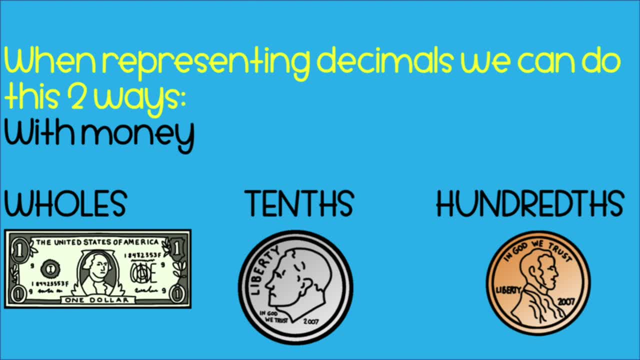 be dollars, tenths would be dimes and pennies would be hundredths. Numbers seem a little less scary as money. somehow, Since we've been working with money for so long, it's easier to answer questions like how many hundredths are in their number. I would like to know how many hundredths are in their numbers. 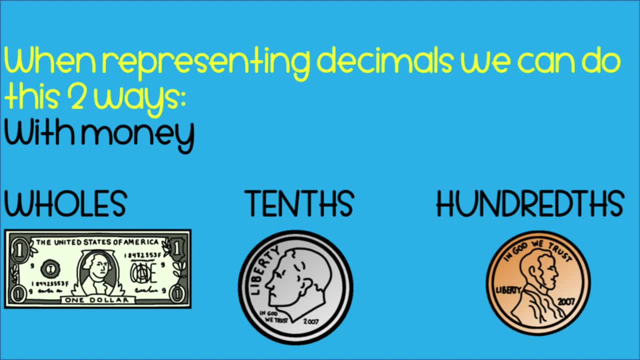 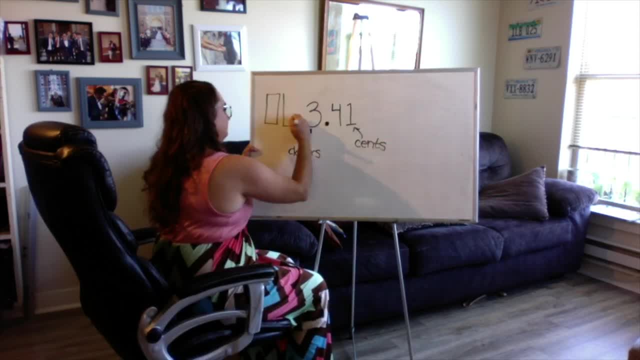 in a tenth. If you think about it as how many pennies are in a dime Ten? Pretty easy, right. Heading over to the whiteboard, if we have the number 3.41,- three represents the number of dollars and .41 is the number of cents, That would be three whole dollars, four dimes or 40 cents. 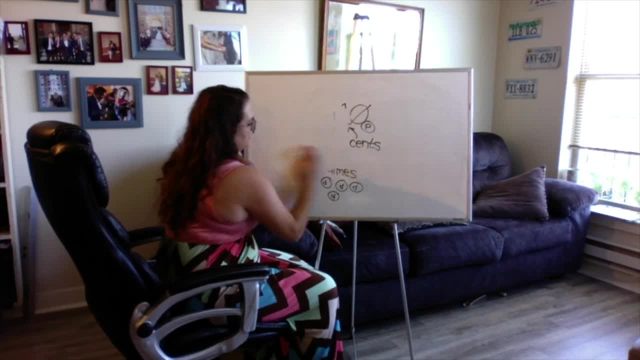 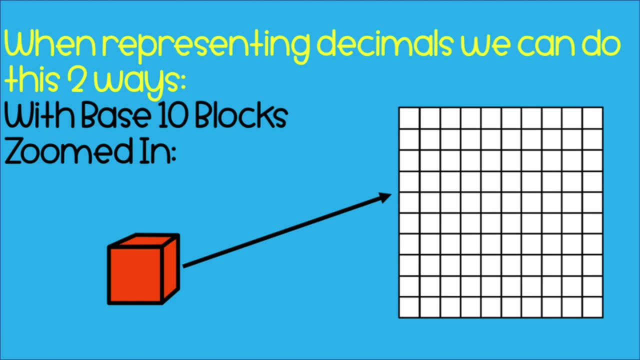 and one penny. If I had a zero there, looking ahead, that zero wouldn't really matter, right? The other way that we can represent decimals is with base 10 blocks. You want to imagine that teeny tiny one from your usual base 10 blocks as if it was zoomed in. I know this looks like a. 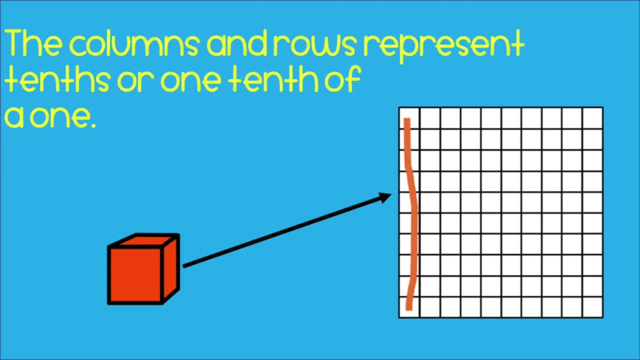 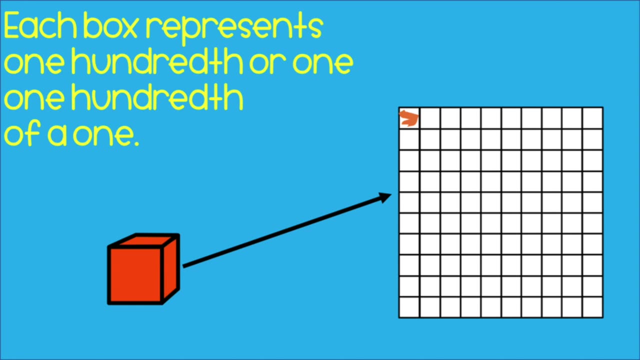 hundred block, but you have to use your imagination. It's zoomed in This: one column of 10 represents one tenth or one tenth of a whole one. Each box represents one hundredth or one one hundredth of one. I don't particularly like this way, but it's really common on standardized tests. 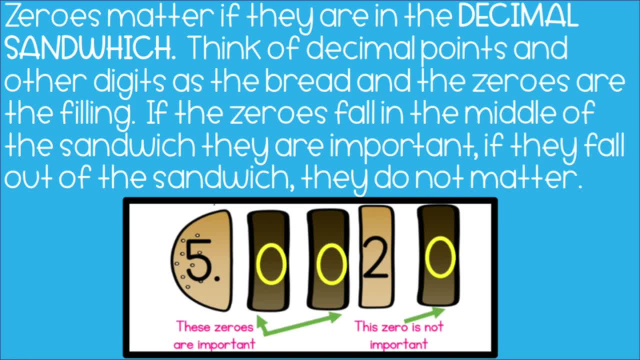 which is why I have it. Probably one of the hardest parts about decimals is understanding which zeros are important and which zeros don't really matter. Zeros matter or count in our decimal place value. if it's in the decimal sandwich, Think of the decimal point and other digits as the bread and the zeros are the. 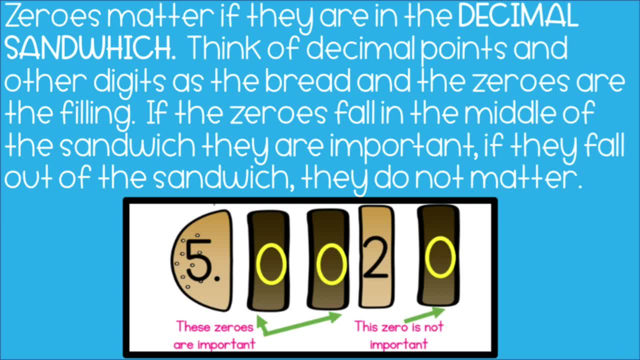 filling. If the zeros fall in the middle of the sandwich, they're important. If they fall outside of the sandwich, then they don't matter. The first two zeros that you see in this diagram matter. They're important. I'm pushing that two to the right. That second zero doesn't really matter. Now let's take a look at this on the whiteboard. 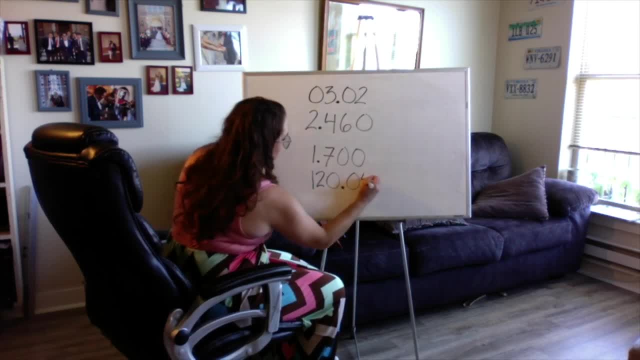 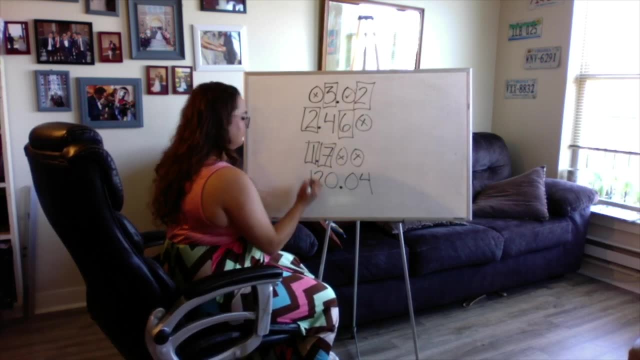 You'll see me writing out a series of numbers. Ask yourself which of those zeros that you see actually matter. I'm putting boxes around my digits that would form my sandwich, and then I'm putting an Xs on the zeros that don't matter and a check on the zeros that do. Whatever is inside my sandwich counts. 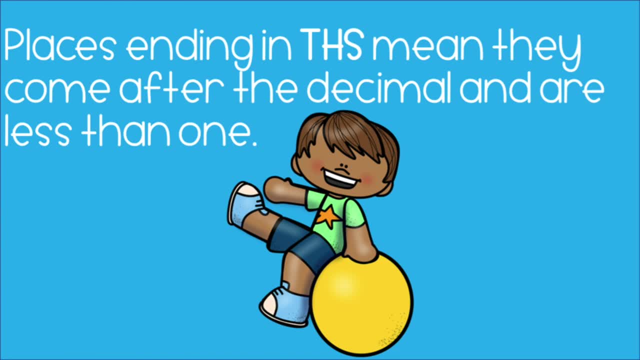 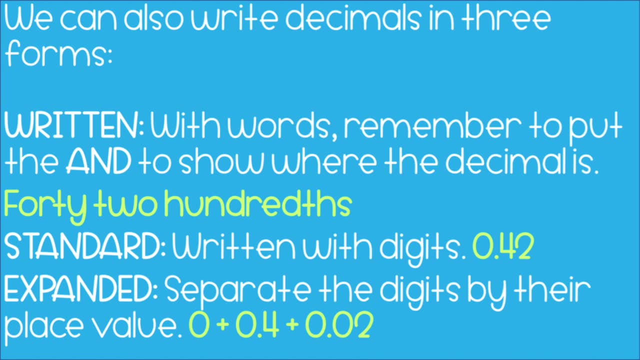 Places ending in fsss mean that they come after the decimal and are less than one. Don't forget to spit. We can also spit, can also write decimals in three forms: written, standard and expanded. and if this feels a little deja vu, it's because we've already talked about this with. 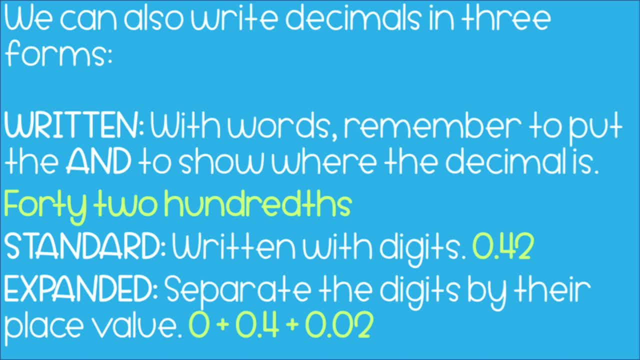 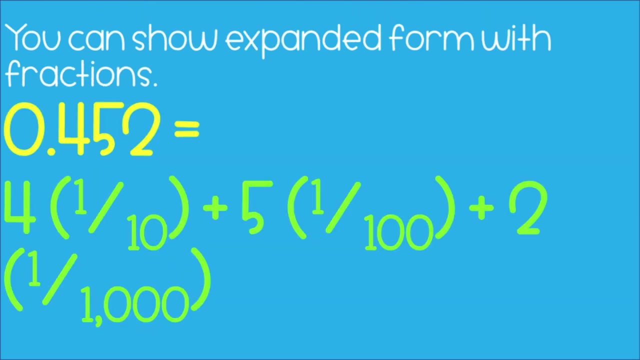 whole numbers and it's the exact same written is with words. remember to put the and to show where the decimal is 42 hundredths. standard is written with digits 0.42, and expanded separates the digits by their place value: 0 plus 4 tenths plus 2 hundredths. you can show expanded form with decimals as fractions. 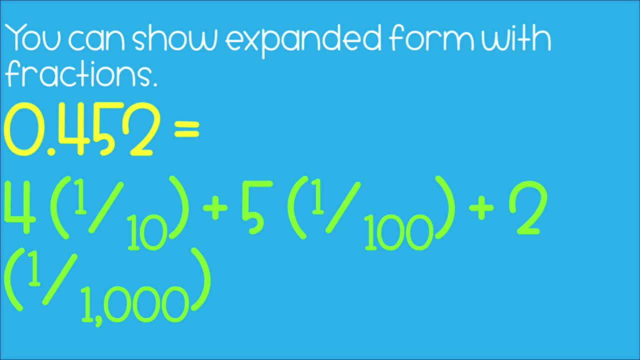 so we have 4 times 1 over 10, plus 5 times 1 over 100, plus 2 times 1 over a thousand. in this particular example that might seem scary, but just remember this is basically just showing the digit and in the place next to it. so the 4 is in. 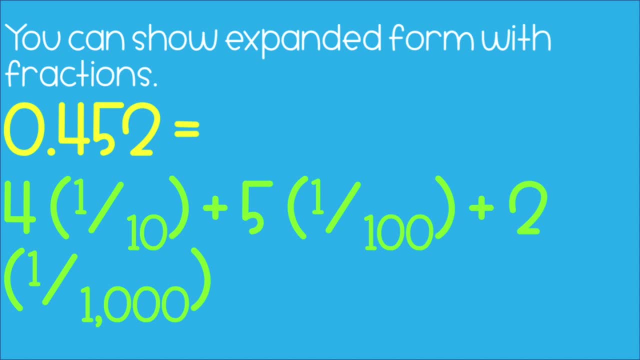 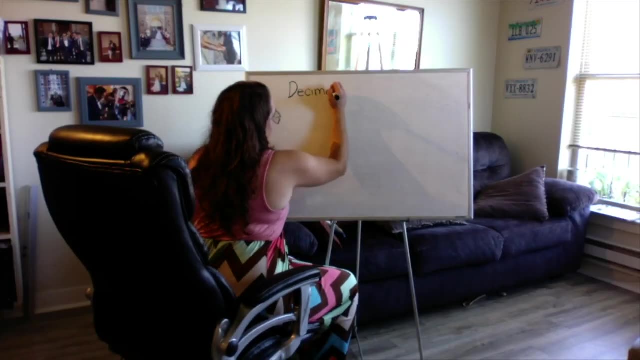 the tenths. so the first digit is the first in the nickel place should be 4 times 1 tenth. the five is in the hundredth place, so it's 5 times 1 hundredth, and so on. let's take a look at this on the right board. like I said, there's two different ways. 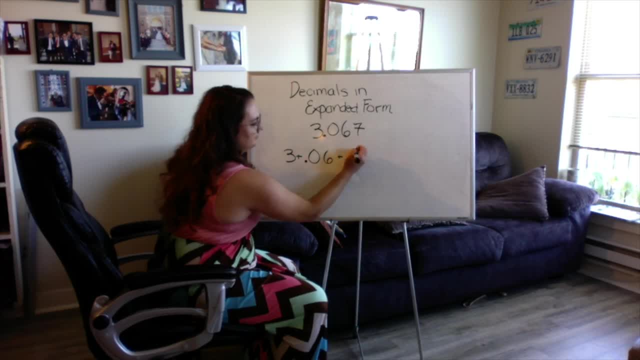 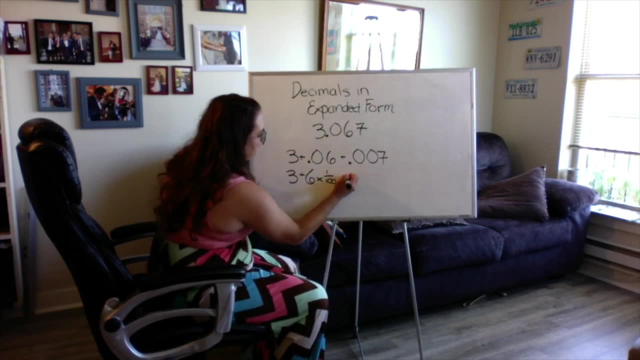 that we can show decimals in expanded form. I recommend writing out the decimal in its place values to begin with, no matter which form you're using: 3 plus 6 hundredths plus seven thousandths. now I'm going to take each of those digits and multiply it by the fraction that represents its place 3. 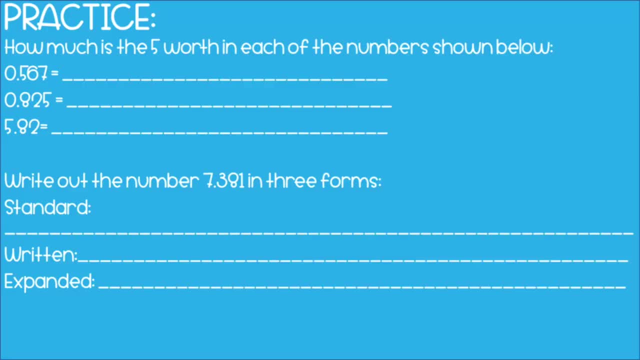 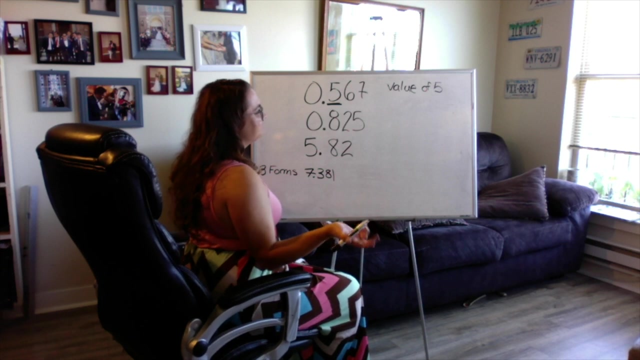 plus seven times one thousandth. Easy, right Now take a moment to do some practice, either by yourself or on the accompanying worksheet. Let's go over these. on the whiteboard I try to underline the digit I'm looking at. I count and tenths, So my first five is equal to five tenths. Be sure to. 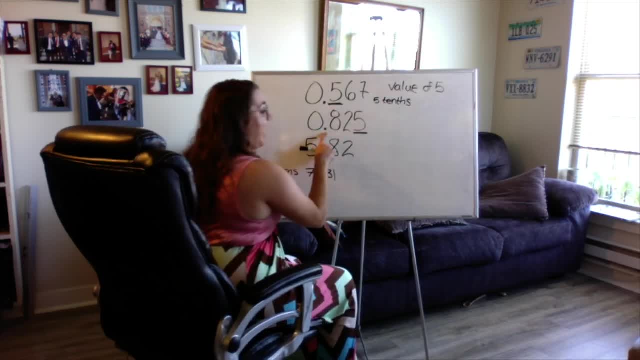 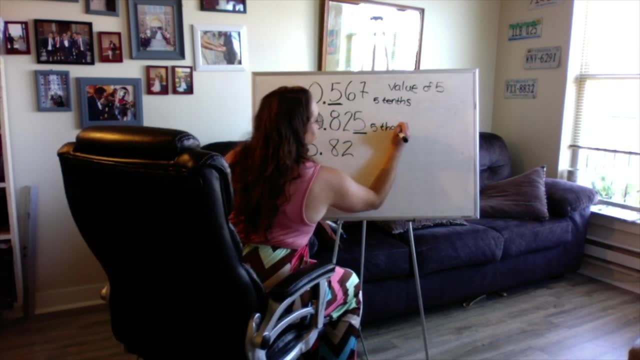 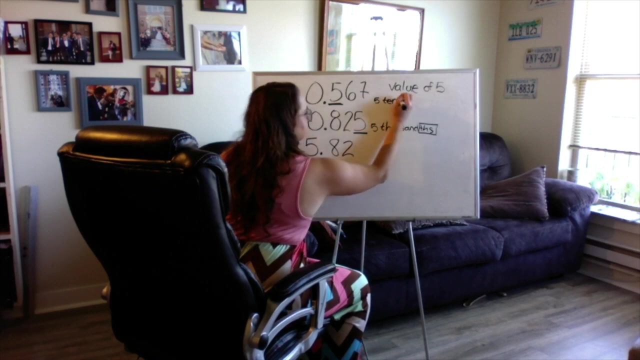 read the question carefully. For this next one, I'm going to underline my five and count, and tenths, hundredths, thousandths. So this number is worth five thousandths. Notice, because we're working with numbers after the decimal. we're ending with that, that spit sound and I'm circling. 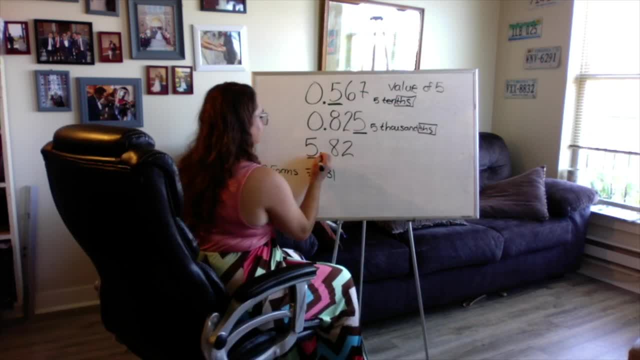 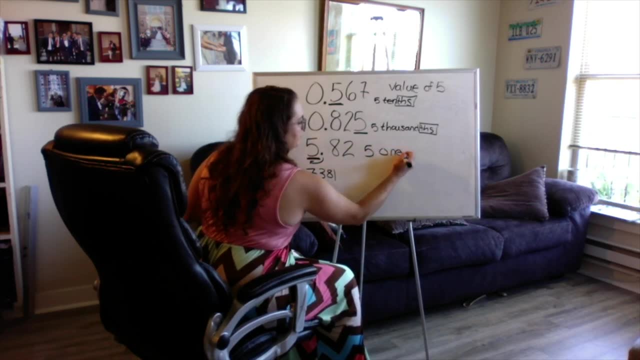 it right here For this last one. the five is my first digit. It's before the decimal, So this is my ones: tens hundredths, so five ones. Our next question is asking us to write the number 7.381. 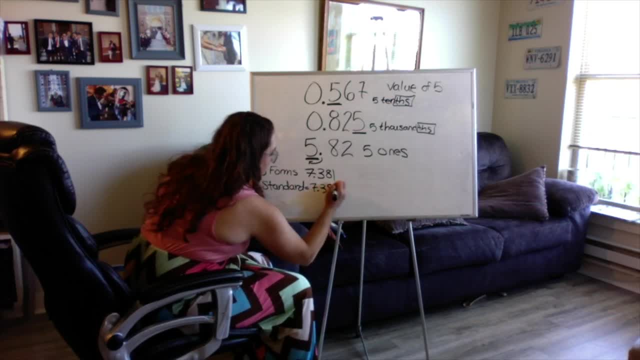 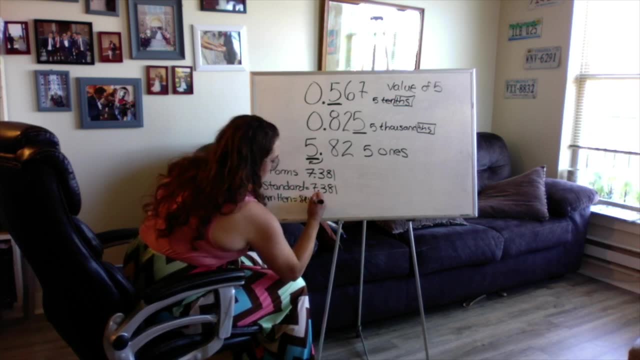 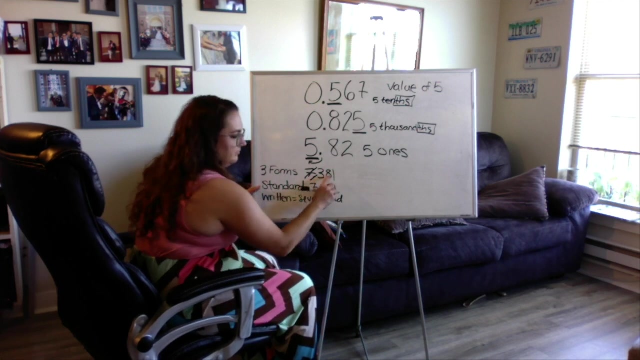 in order. So the first way is, just as it's written standard form, with digits seven and three hundred eighty-one thousandths. I try to read it out loud to help me with my written form, which is what I'm writing with words. You'll also see me cross off each of the digits to make sure that I've 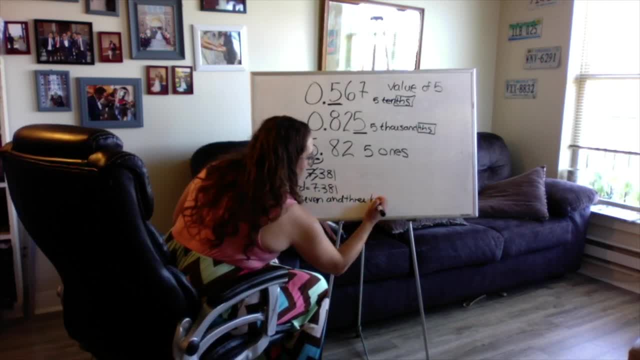 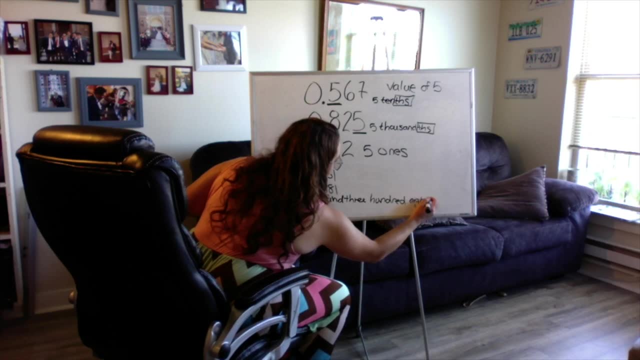 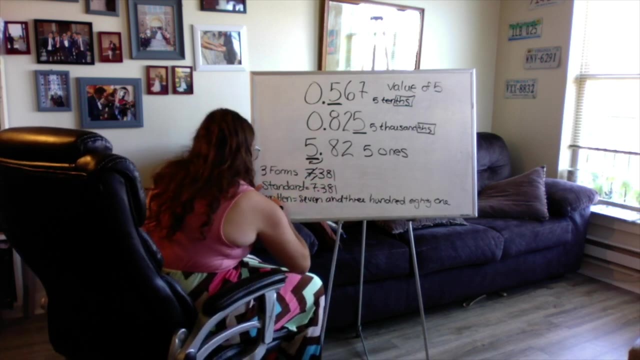 accounted for them in my number. You want to make sure that you're using the name of the furthest digit to the right. In this case it is thousandths. So we have seven and three thousandths. I have seven and- and is my decimal- three hundred eighty-one thousandths, because I have 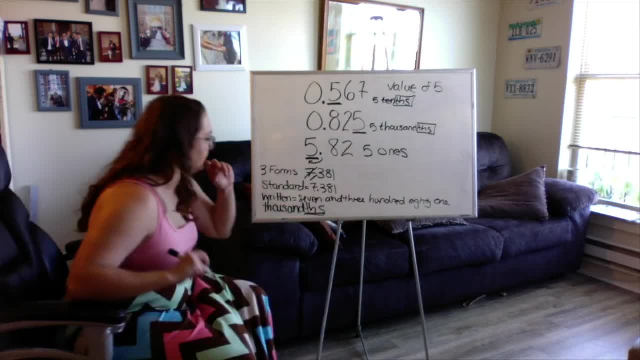 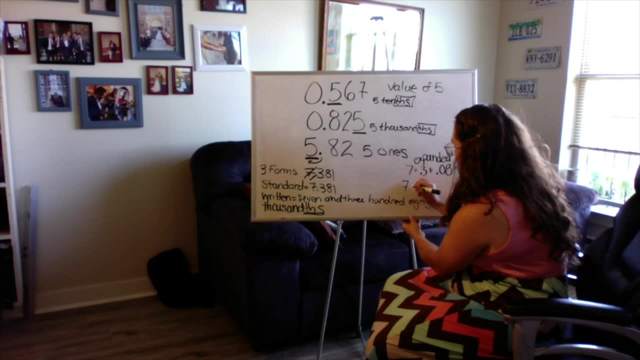 tenths, hundredths, thousandths. Now let's take a look at this in expanded form. You'll see me start by separating my digits based on their place value. That's one way to write it. The other way to write it is to include it multiplied by the fraction. So I have seven plus three times one. 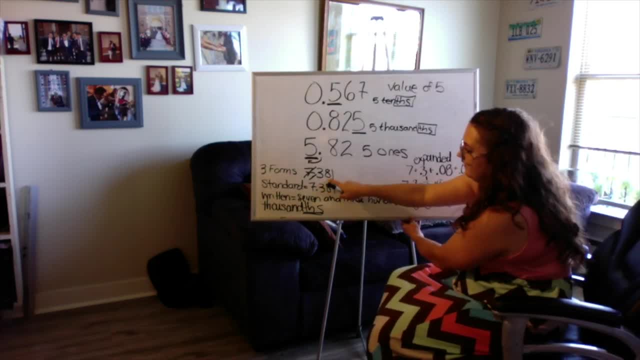 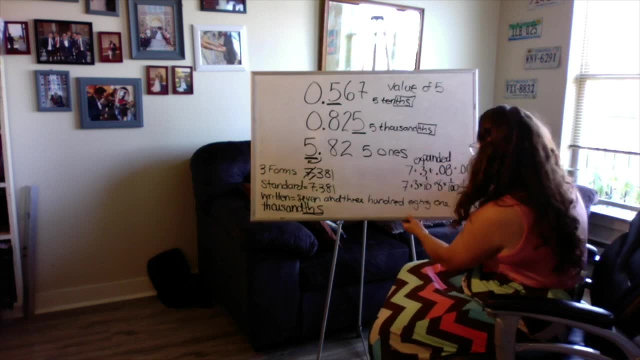 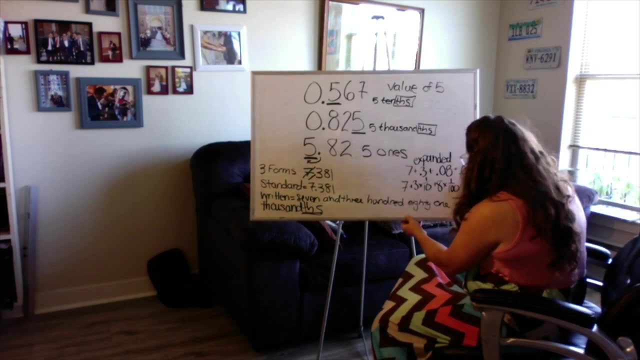 tenth, because my three is in the tenths place, plus eight times one over a hundred, because I have my eight in my hundredths place, Plus one times one over a thousand, because my one is in my thousandths place. It looks kind of scary, but just remember you're multiplying it by the fraction that represents the place. 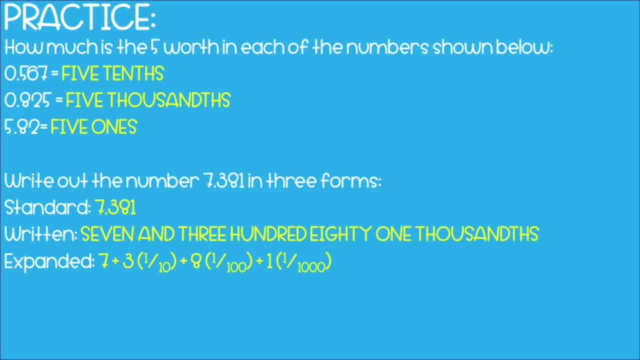 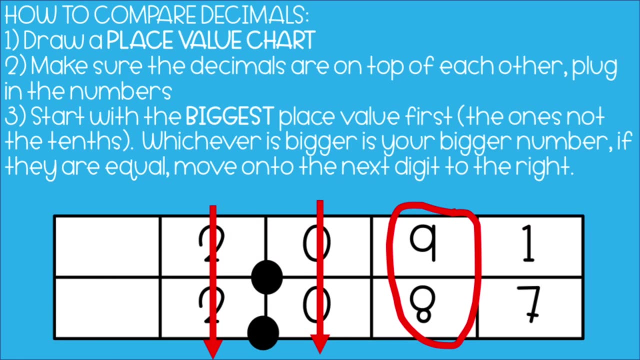 that that digit is in. Always feel free to pause if you need more time, but the answers are here for you to check. if you need them Now, let's use something we talked about in our last lesson to compare decimals, or to use those greater than, less than and equal. 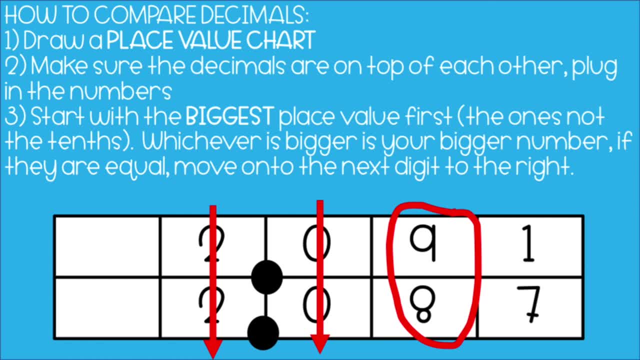 to signs to show which decimal is bigger. The first thing you need to do is draw a place value chart. Don't be intimidated by the word place value chart. it's just a table or a big rectangle with a bunch of smaller boxes inside. The next thing you need to do is make sure your decimals are drawn on top of each. 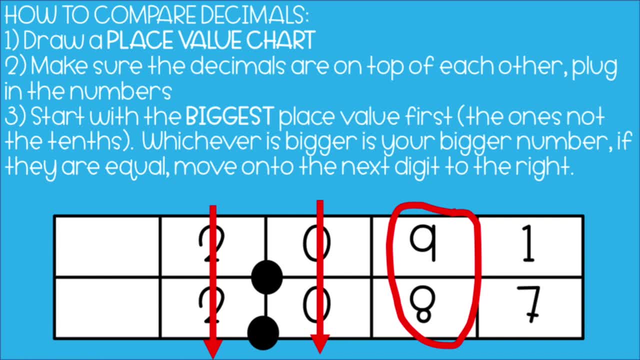 other. I like to think about this as a snowman. My decimals should stack on top of each other to form a kind of snowman. Now plug in your numbers, making sure the decimal is in the right spot in your number. Start with the biggest place value first In this particular. 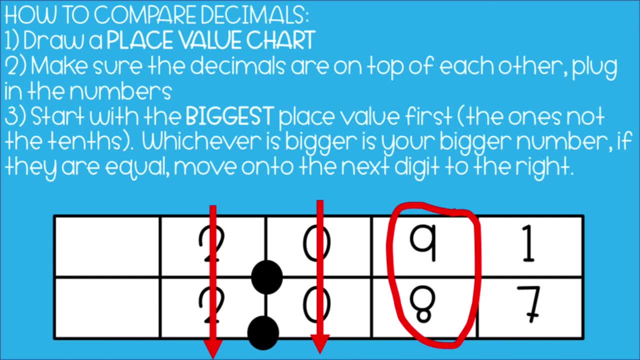 example, the ones are my biggest place value. Whichever number is bigger, that's your bigger number. If they're equal, then you move on to the next digit. So in this one I crossed off my twos because they're the same in my ones place. I then move to my tenths, My zeros. 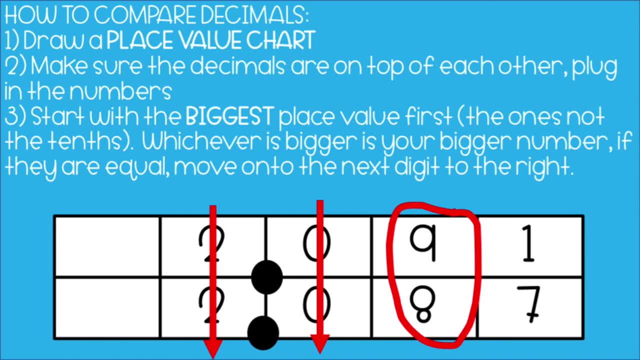 are the same. I crossed them off. so now I move on to my hundredths. My top number, 2.091, is bigger because 9 is bigger than 8.. It doesn't matter that the next one has a 7,. I'm looking. 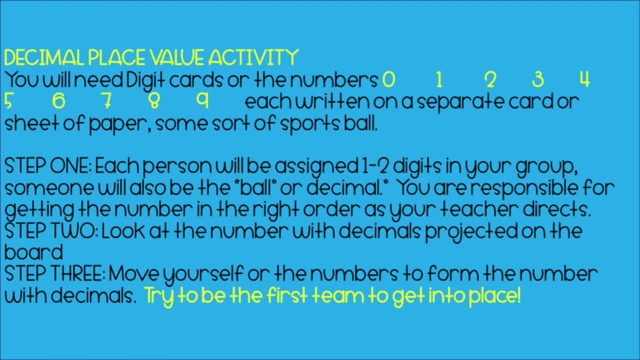 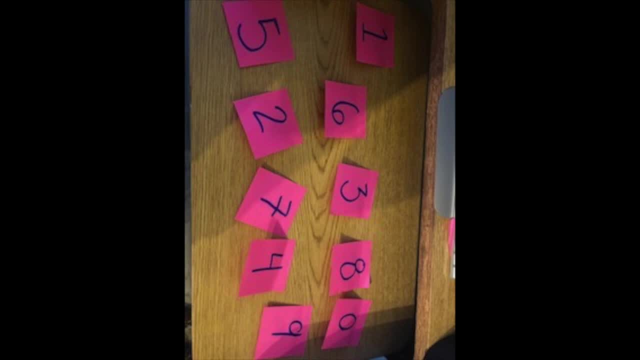 for the first biggest number. Now it's time for a decimal place value: activity. For this activity you're going to need, ideally, post-it notes with the digits 0, 1,, 2,, 3,, 4,, 5, 6,, 7,, 8, 9 written on them. Don't have 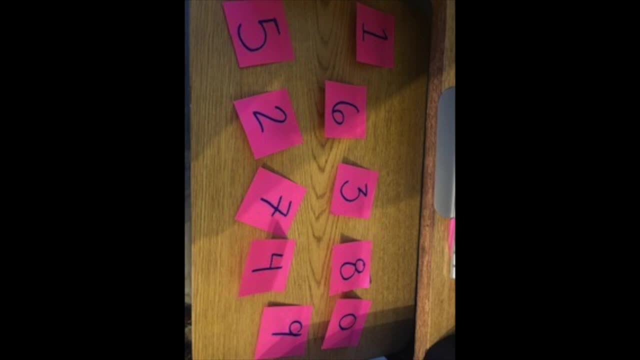 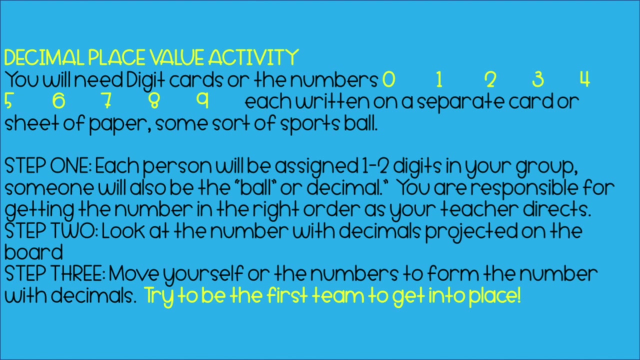 post-it notes. That's okay. You can write it on index cards or scrap sheets of paper. The important thing is that you're able to move the digits around. The next thing you're going to need is something to represent the decimal. This could be a sports ball. it could. 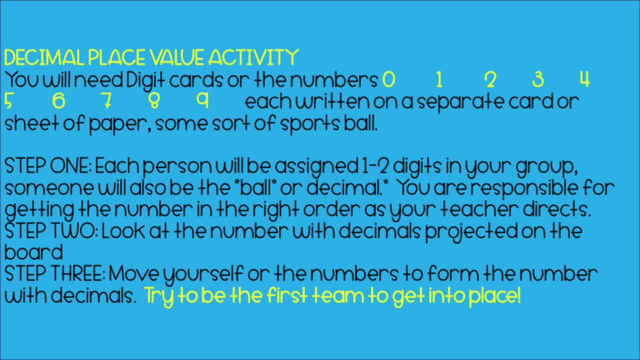 be an M&M, it could be a football, it could be a basketball, it could be a basketball. it could be a rock. you found outside Just something that will represent that decimal. I'm going to show a picture of something, either a form of a decimal or an image that. 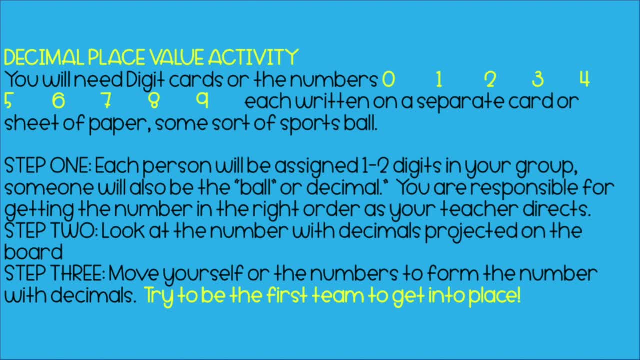 represents a decimal and your job is to take those digits and put them in the right order to form the correct decimal before the answer appears. Note: you can always pause the video if you need more time. Good luck, and I know you're going to kick some math, gluteus maximus. 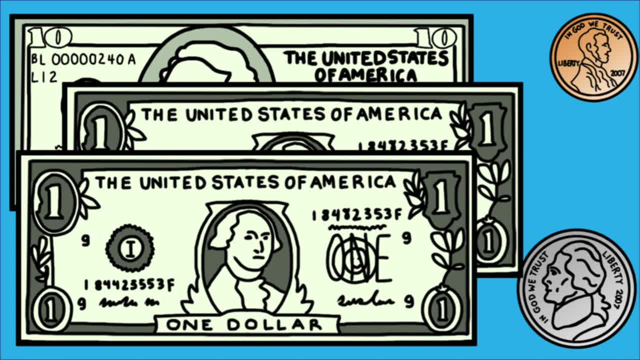 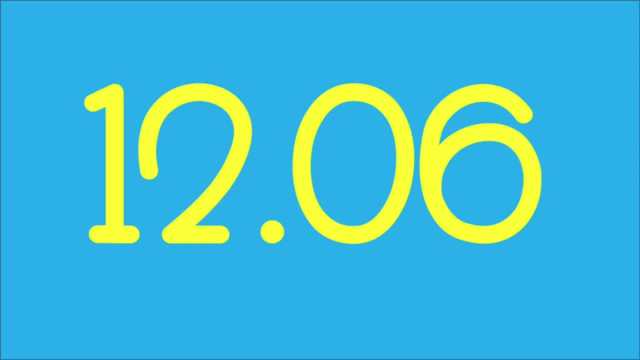 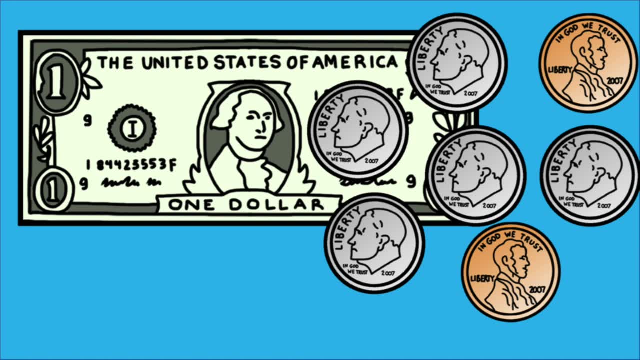 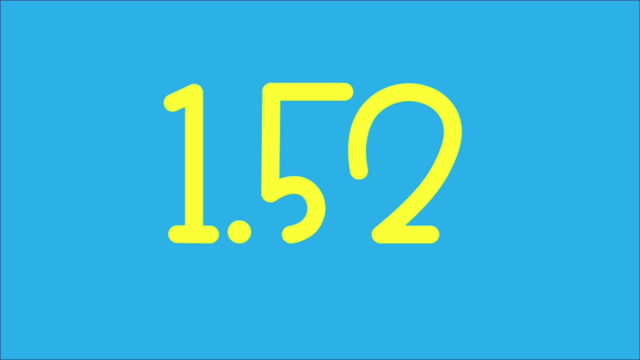 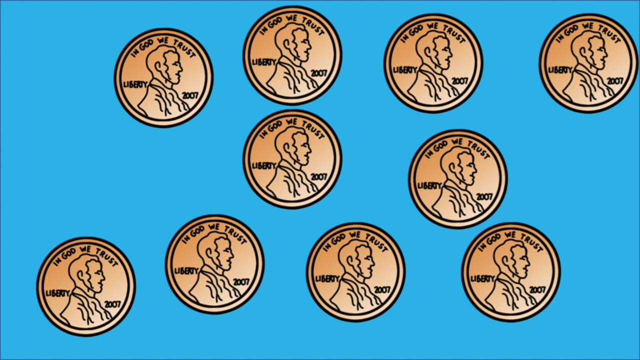 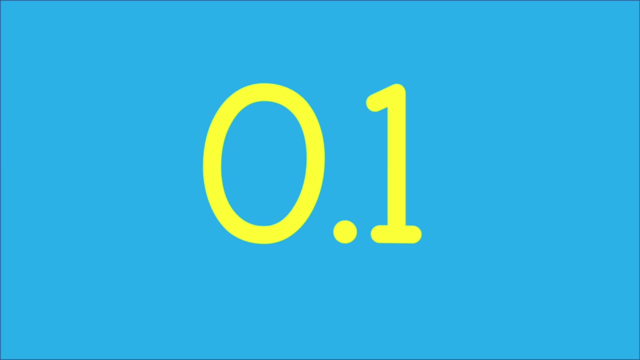 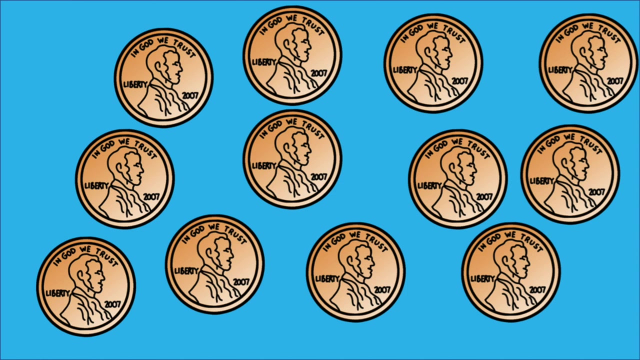 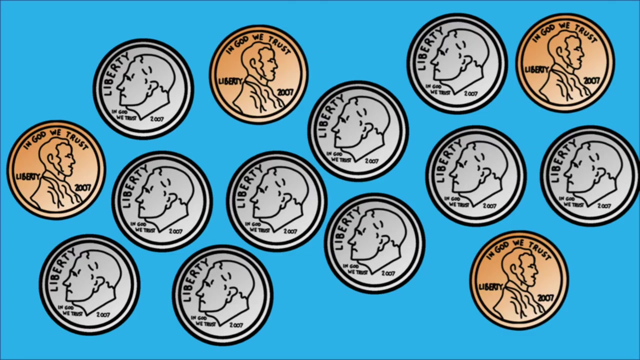 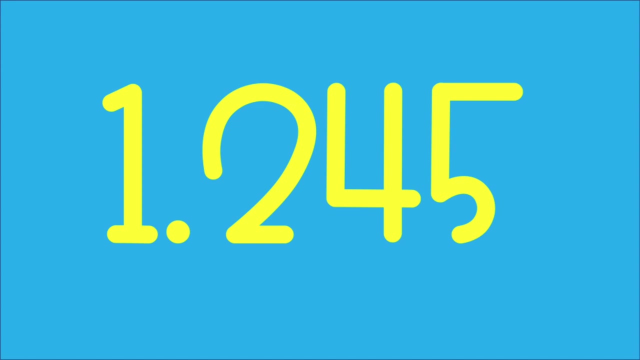 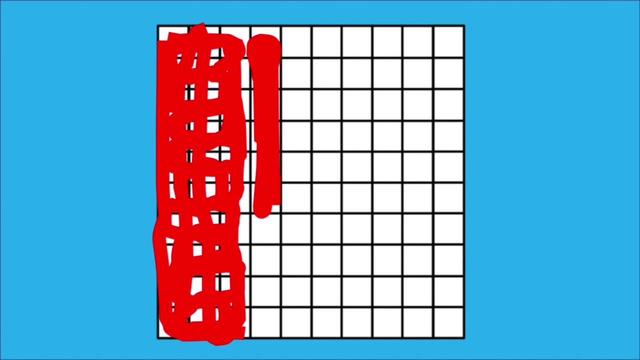 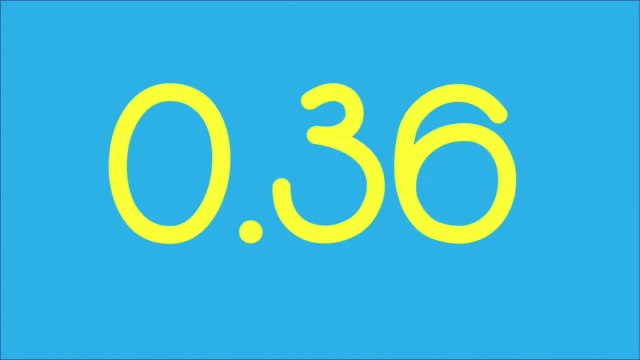 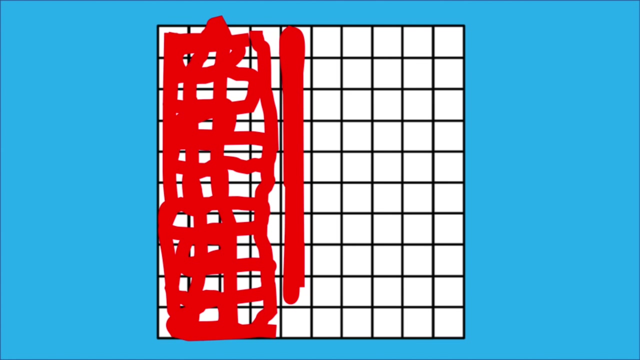 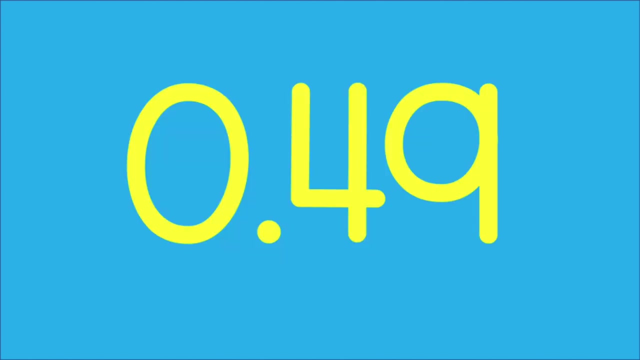 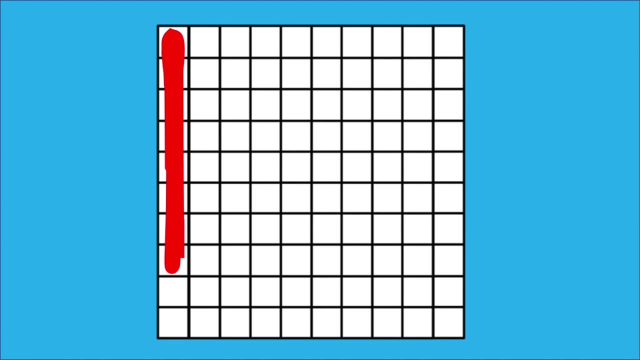 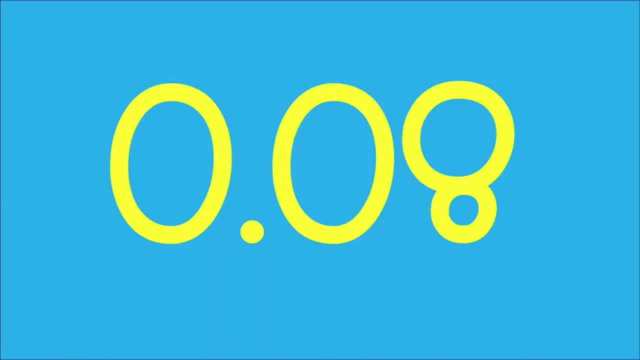 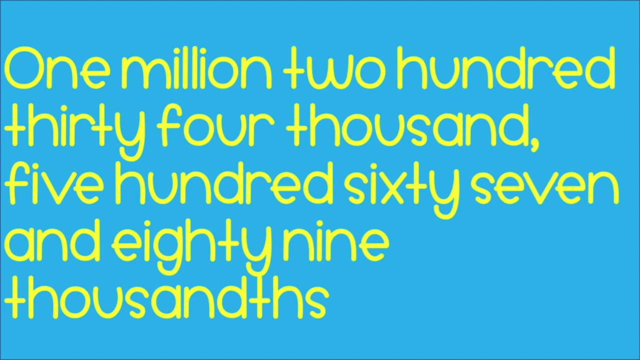 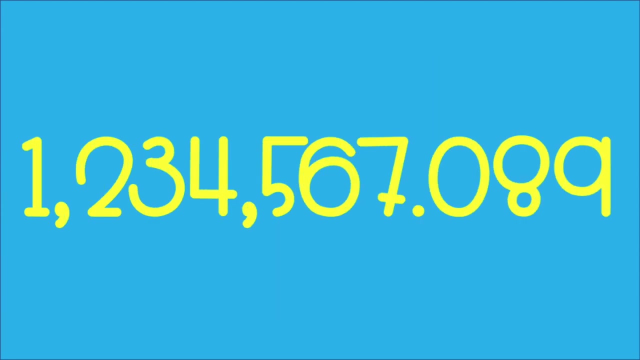 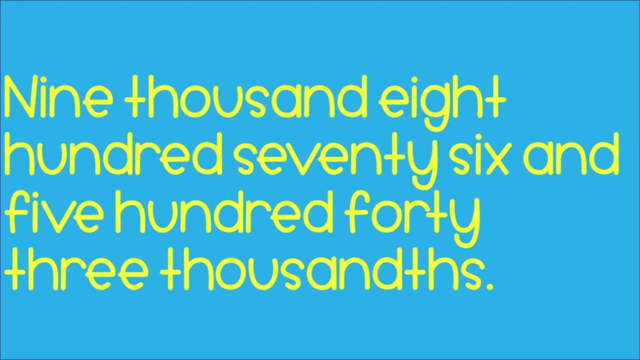 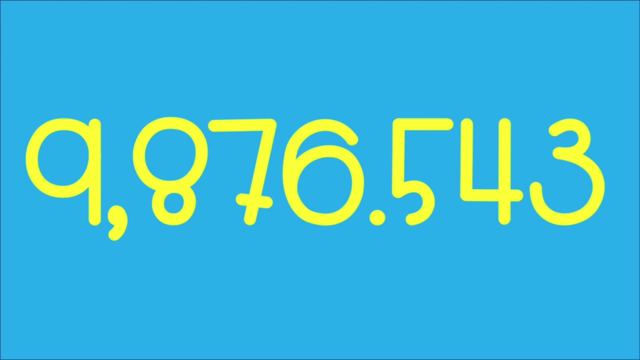 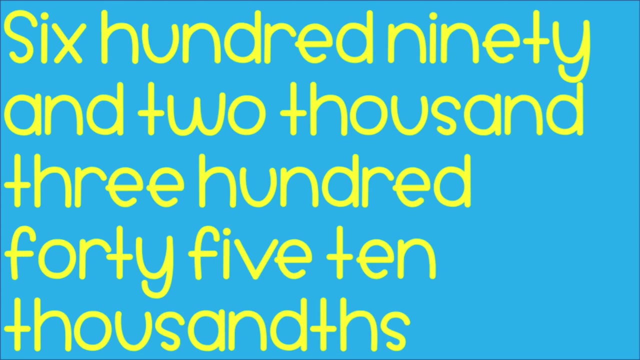 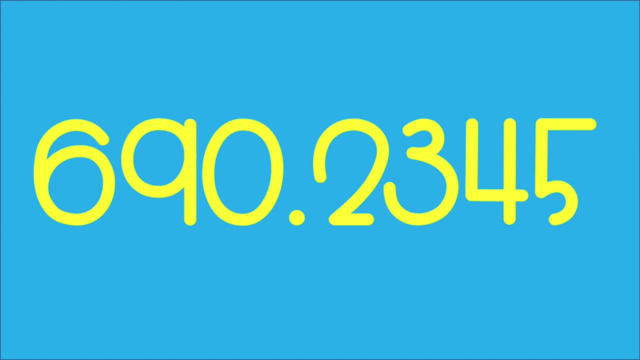 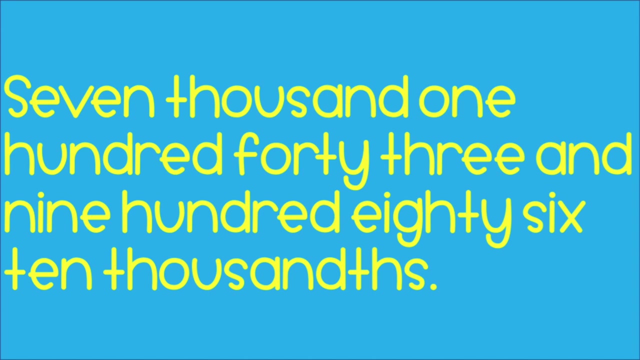 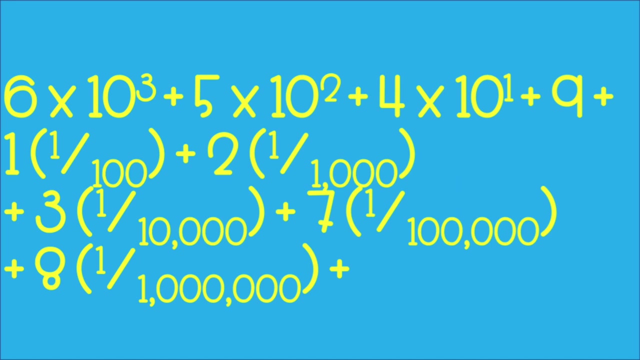 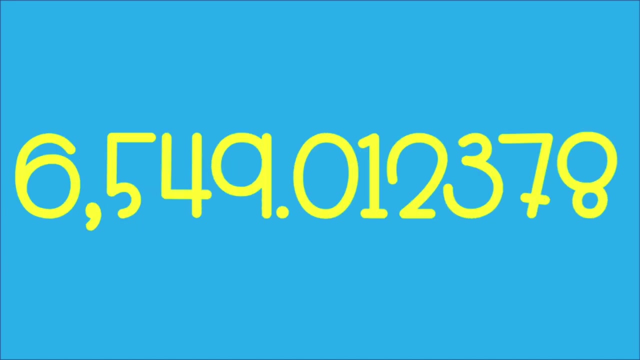 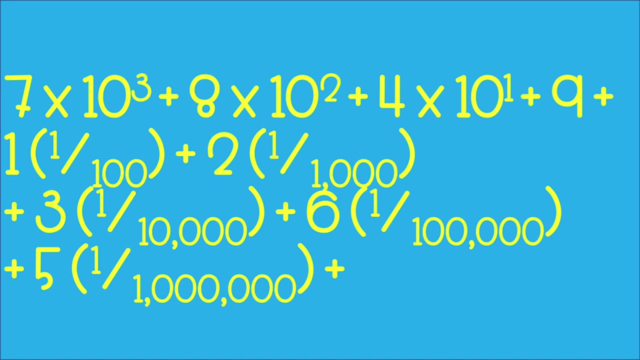 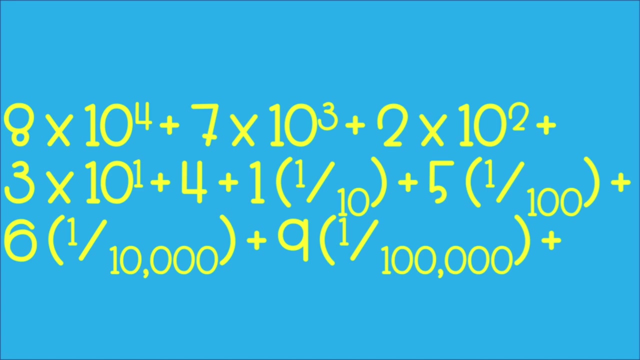 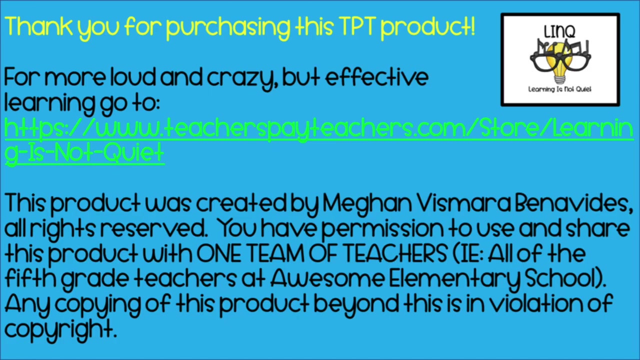